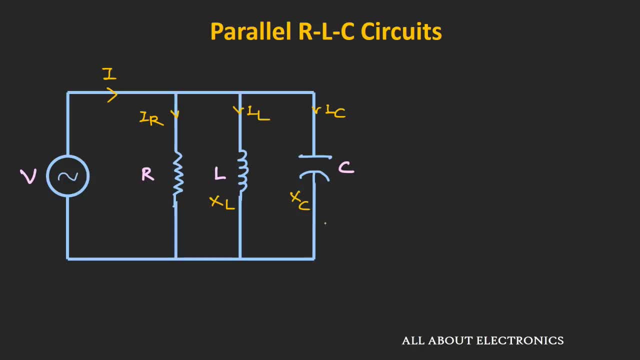 this capacitor. So now, whether the circuit is series RLC or a parallel RLC, the resonance condition remains the same. That means when the XL is equal to XC, or we can say that if inductive reactance that is equal to the capacitive reactance, then the circuit will be. 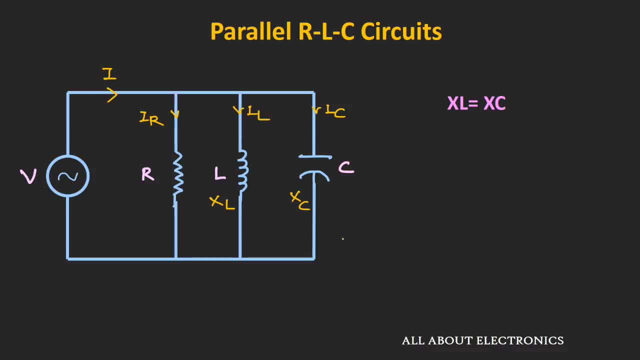 in a resonant condition And during the resonance, if you see, the impedance of the circuit will be purely resistive. That means the voltage and current will be in a phase. Also, at resonant condition, if you see, the impedance of the circuit will be maximum. So at resonant condition the current that 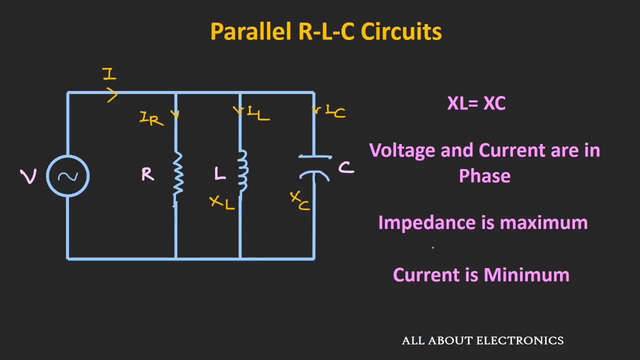 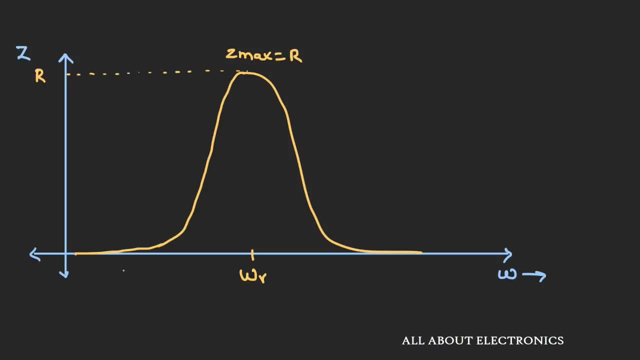 is supplied by the voltage source will be the minimum, Because the impedance of the circuit is maximum. So these are some of the points which you see at a resonant condition. So now this is a plot of impedance versus the frequency for a parallel RLC circuit. So as you can see here at resonant frequency, 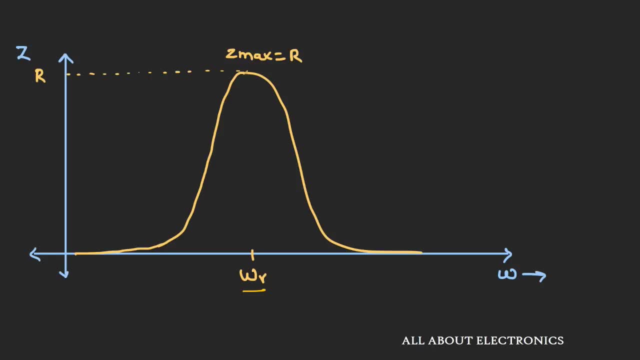 the impedance of the circuit is maximum And as we move away from this resonant condition, the impedance will reduce. Now, if you see, at, ω is equal to 0, the XL term will be 0. So the overall impedance of the circuit will. 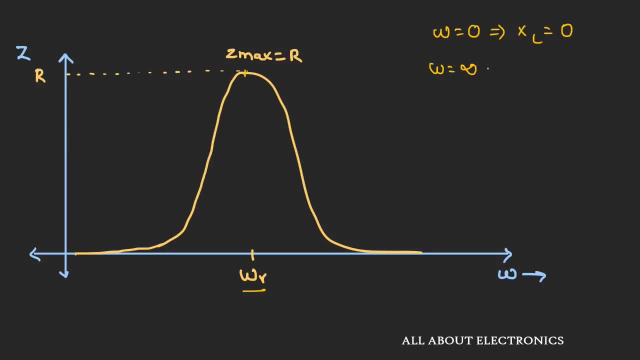 be 0.. Similarly, at ω is equal to ∞. if you see this term, XC, that is equal to one, over ΩC, which is equal to 1.. will be also zero. So that is the reason. at lower and higher frequencies, the impedance. 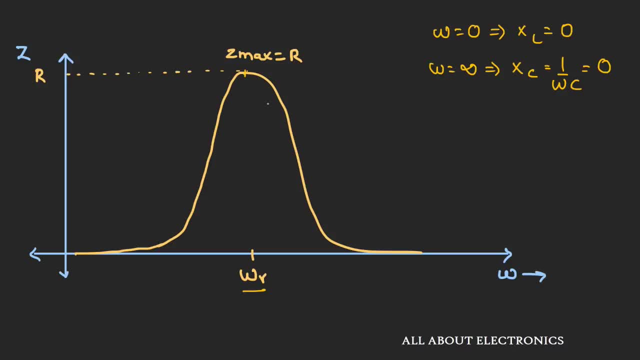 is minimum, While at resonant condition, if you see, the impedance will be the maximum And the maximum value of this impedance will be R. So at resonant frequency the impedance of the circuit will be purely resistive. Similarly, if you see the current versus frequency, 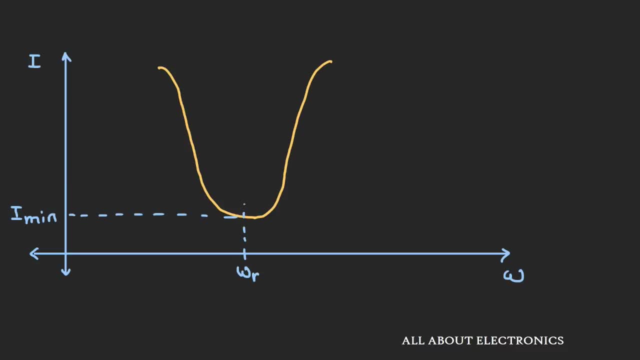 curve. it will look like this: At resonant condition, the current that is flowing through the circuit will be the minimum. So as you move away from this resonant frequency, the current will start increasing. So now, if you see this current versus frequency curve, 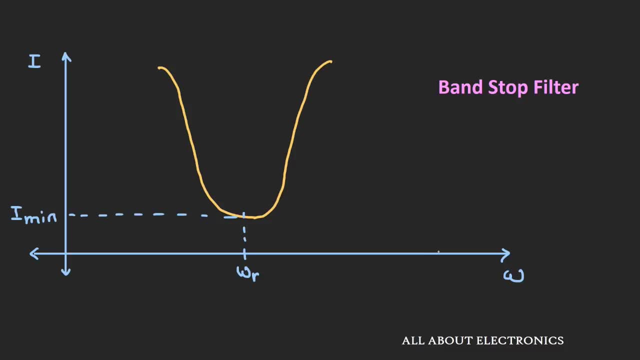 for this parallel RLC circuit it looks like a band stop filter, Because it rejects some frequencies and passes all other frequencies, While in case of a series RLC circuit we had seen that it acts like a band pass filter, as it passes few frequencies and rejects all. 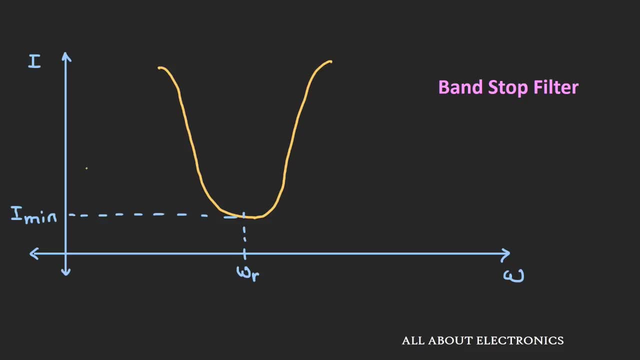 other frequencies, And that is the reason this circuit is parallel. RLC circuit is also known as the rejector circuit, While the series RLC circuit is known as the acceptor circuit. So now let's derive the expression for this resonant frequency mathematically. So now let's once again assume that the current, that 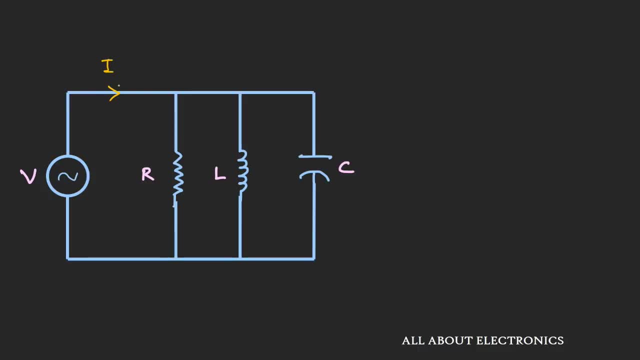 is supplied by this circuit, is I Now here? this current? I is nothing but a RMS current, So instead of writing this as I RMS, I am simply writing it as I, And similarly, the voltage here that is indicated as V is also a RMS voltage. 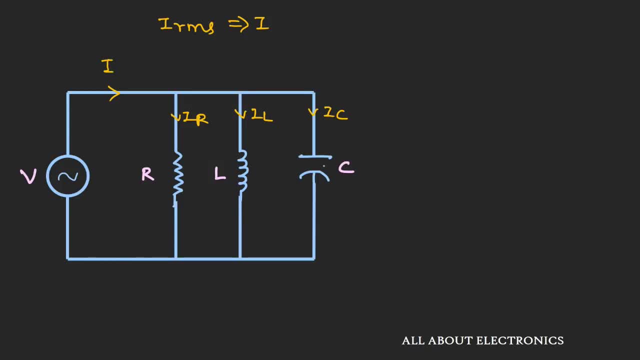 So assume that the current that is flowing through this resistor, inductor and capacitor are I R, I L and I C respectively. So now, if we apply a KCL at this node, then we can write it as I is equal to I R plus I L plus I C, Or we can write it as V over. 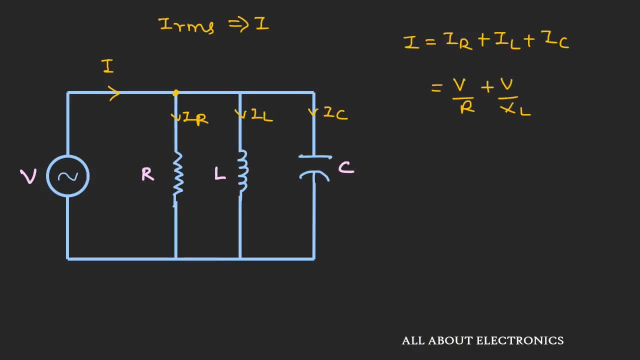 R plus V over X L plus V over X C, That means V into 1 over R plus V over X L plus V over X C, That means V into 1 over R plus V over X L plus V over X C, That means V into 1 over. 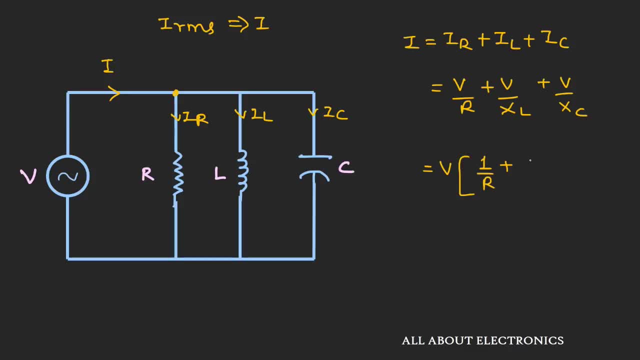 R plus. Now XL is nothing but a 1 over j omega L, And similarly the XC is nothing but a 1 over j omega C. So we can write it as j into omega C. So further we can write. 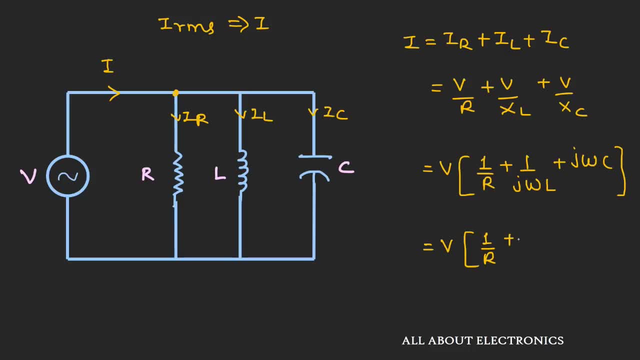 it as 1 over R plus j into omega C, minus 1 over omega L. Now, if you see this term, this term is nothing but an inverse of impedance, Which is known as inverse of impedance. So this is known as admittance And it is denoted by symbol Y, So we can write this equation: 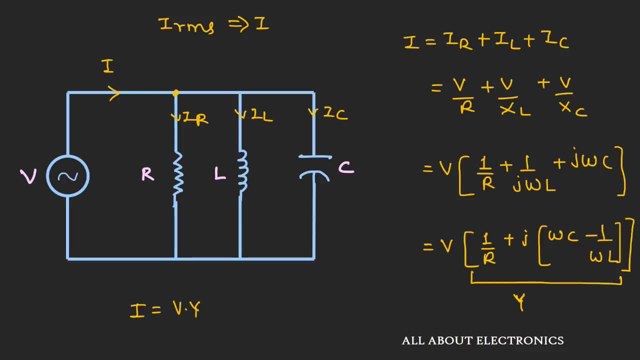 as I is equal to V into Y. Now, at resonant frequency, the current that is flowing through the circuit is minimum. And to get a minimum current, this Y should be also minimum. And to get the minimum value of this Y, this omega C should be equal to omega L. So when omega 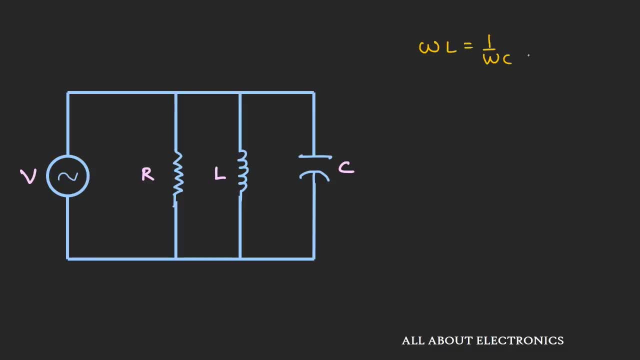 L is equal to 1 over omega C, Then the value of Y is nothing but 1 over R, And we get a value of current I as V over R. So, at resonant frequency, the value of admittance is minimum, Hence the value of impedance. 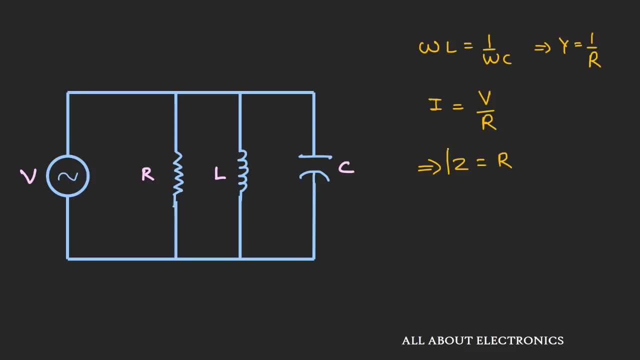 is maximum, And this maximum value of impedance is nothing but a resistor R. So this condition- omega L is equal to 1 over omega C- is known as the resonant condition. So now let's find out the frequency at which this resonance is happening. So as 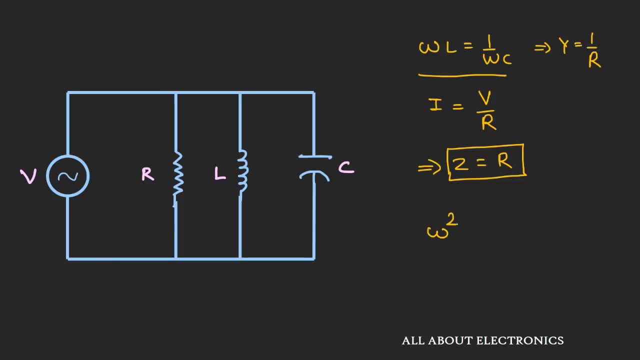 O, equal to 1 over omega c. So we can write it as omega square, that is equal to 1 over LC, Or we can write it as omega, that is equal to 1 over under root LC. So this is the resonant frequency in a. 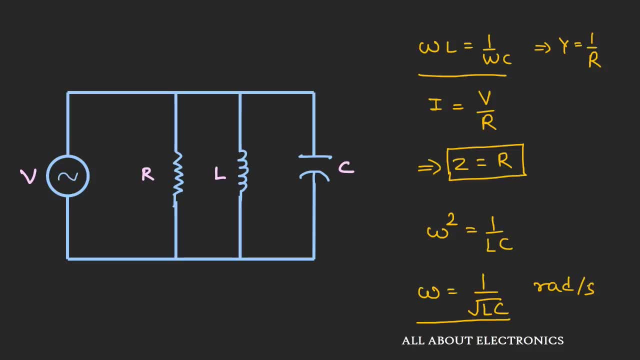 radian per second at which this resonance is happening, Or simply if we write it in terms of the frequency, then we can write it as a F that is equal to 1 over 2pi under root Four generator. So this is the equation for the resonant frequency. 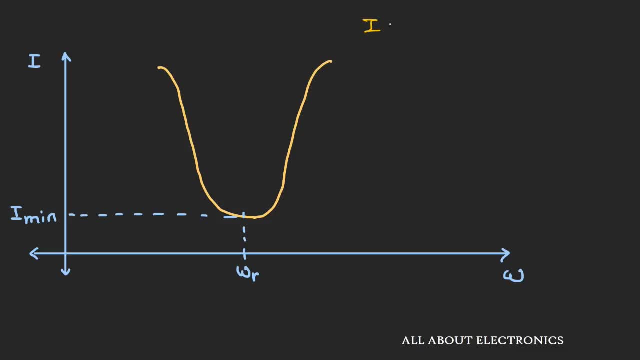 And at this resonant frequency the current that is flowing through the circuit is nothing but V over R. That means the circuit will be purely resistive circuit. So now, if you see at ω is equal to zero, the value of xl will be zero. 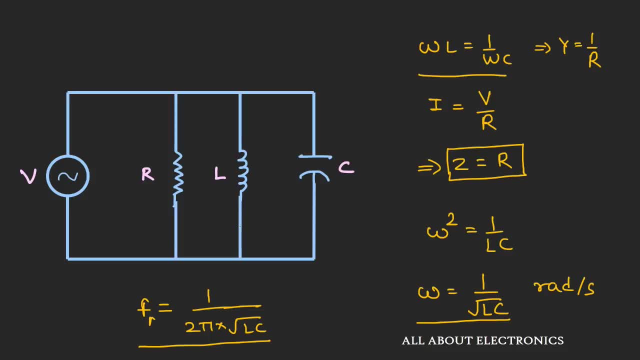 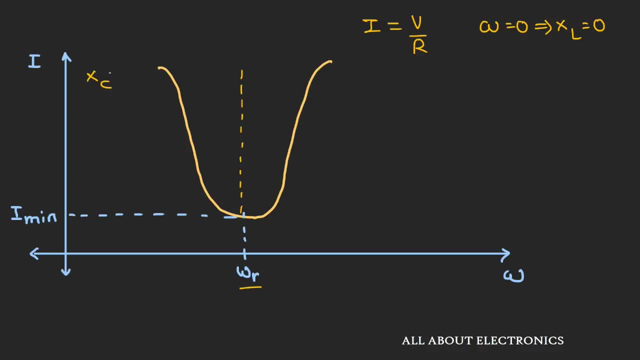 So this inductor will act as a short circuit And entire current will flow through that inductor. So for the frequencies which are lesser than ωR, this xc will be greater than xl, As xc is given as 1 over ωc. 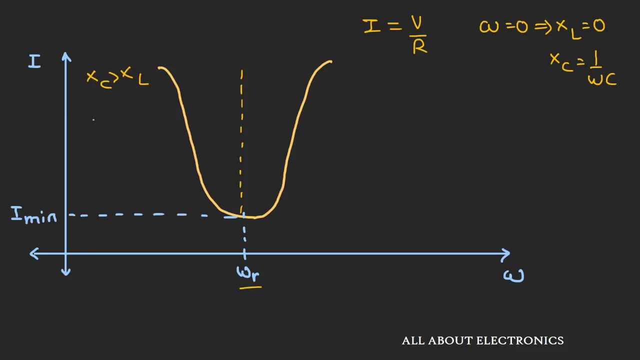 And circuit will behave as an inductive circuit. That means this: current I lags the voltage, While at higher frequencies, if you see, let's take a frequency ω, that is equal to infinity, the xc is nothing but zero. So for higher frequencies, if you see, 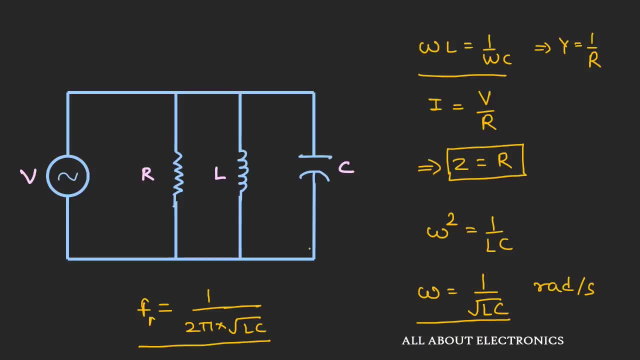 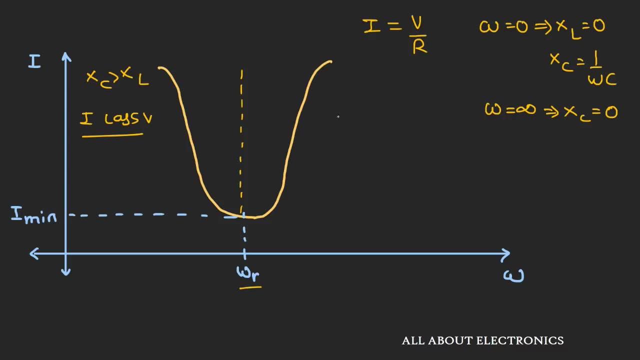 this capacitor will act as a short circuit And entire current will flow through that capacitor. So at higher frequencies this capacitive reactance is dominant, And at higher frequencies this current leads the voltage. So for the frequencies which are lesser than this resonant frequency, the behavior of the 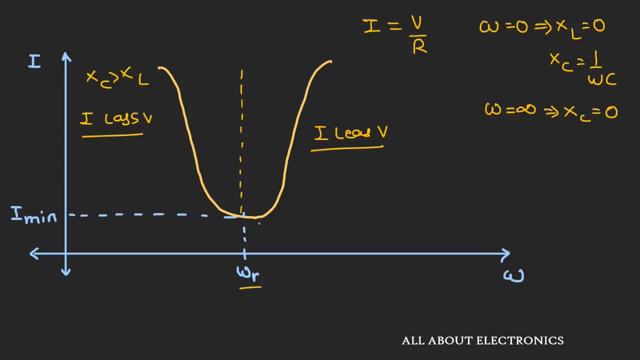 circuit will be inductive And for the frequencies which are higher than this resonant frequency, the behavior of the circuit will be capacitive. So now in the last video we had seen, if you see, this capacitor will act as short. 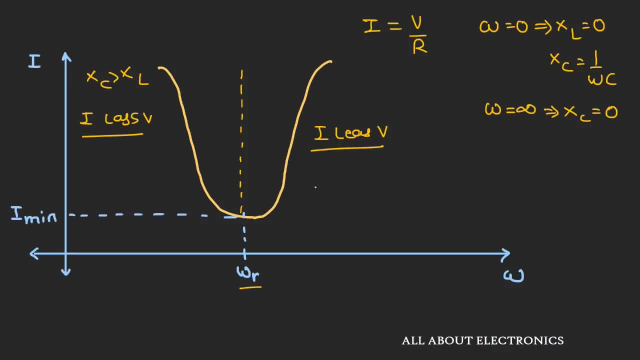 circuit, that to define the sharpness of this resonant curve, the two parameters are used, which are quality factor and bandwidth. So now let's see them one by one. So first let's talk about the quality factor. So, as you can see, here we have three different. 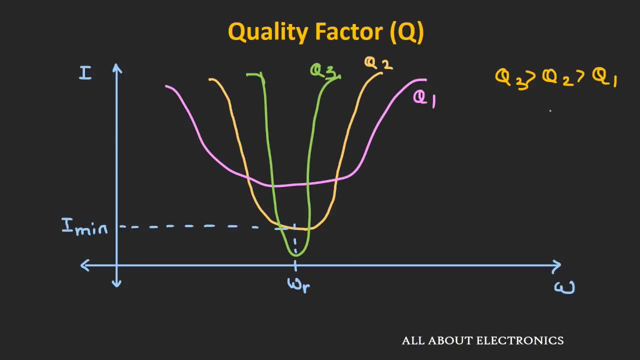 curves for the different value of Q. So now, as the value of this quality factor for the circuit increases, the sharpness of the curve also increases And the resonant curve is getting narrower and narrower. So we are able to reject one particular frequency. 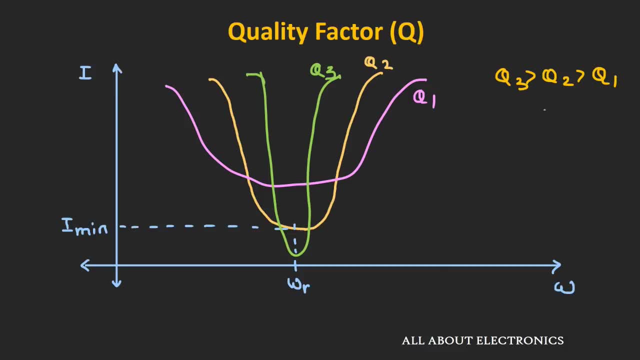 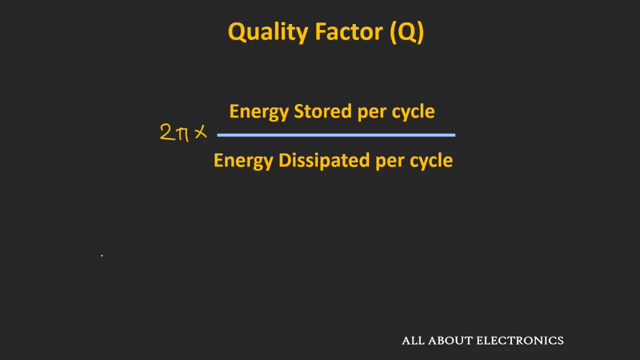 very precisely. And as the value of this quality factor reduces, the curve is getting wider and wider. So instead of rejecting one single frequency, it will reject many other frequencies as well. So now let's find out the equation for this quality factor in terms of the circuit components. So now, in the last video we had seen that 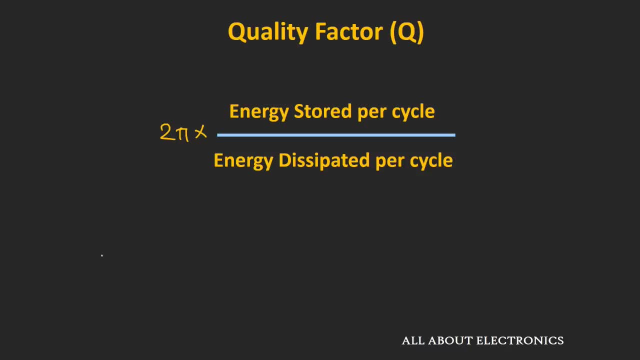 the quality factor can be defined as 2Φ into the maximum amount of energy that is stored across either inductor or capacitor, geared by the energy that is dissipated across the resistor. So we can also write this equation as ω into energy that is stored per cycle geared. 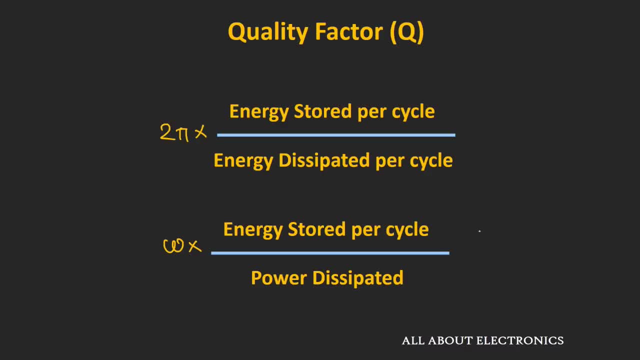 by the power that is dissipated across the resistor. Now we know that the energy across the inductor or capacitor can be given as ½ Li², that is equal to ½ Cv². This term defines the energy that is stored across the inductor And this term defines the energy. 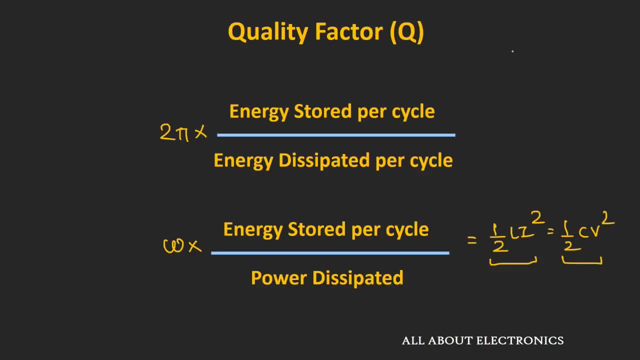 that is stored across the capacitor. Now, here, this current I is nothing but a maximum current. It is flowing through the circuit. So now, if we write this equation in terms of the RMS values, where Irms is nothing but Imax geared by root 2. And Vrms is nothing, 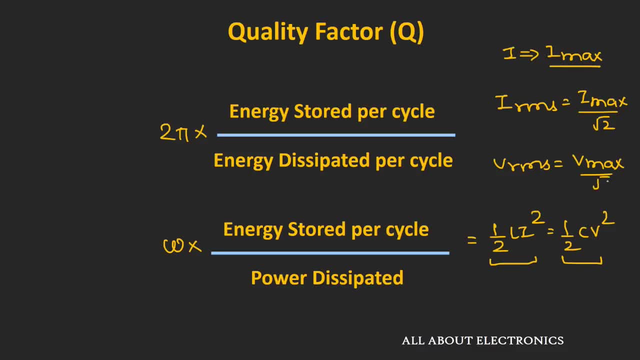 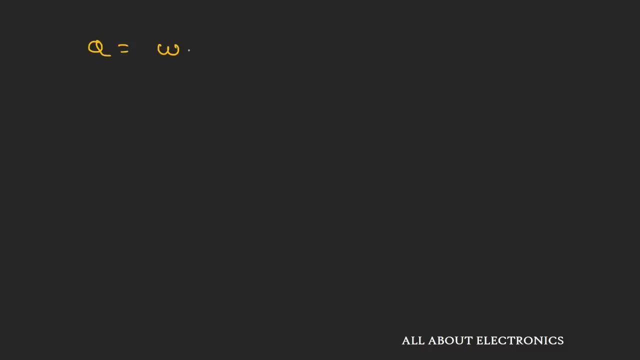 but Vmax over root 2.. Then we can write them as L, ln, Irma square. that is equal to Cv, V rms square. So now this Q, we can write it as a Rm, So omega, into C, into V? rms square. that is the energy that is stored across the 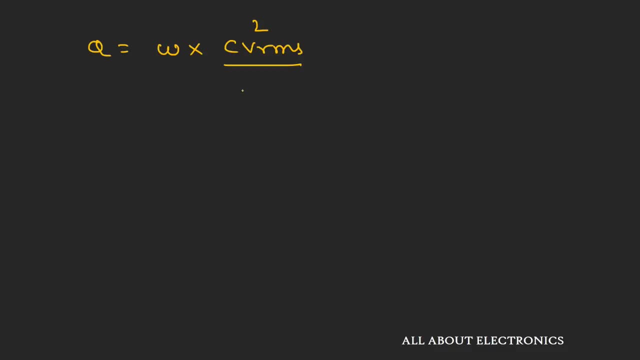 capacitor there by the energy that is dissipated, or a power that is dissipated across the resistor, which can be given as I, rms square into R, or we can write it as a omega into C, into V: rms square there by V, rms square there by R. so we will get omega into C into R. now we know that the X C can be written. 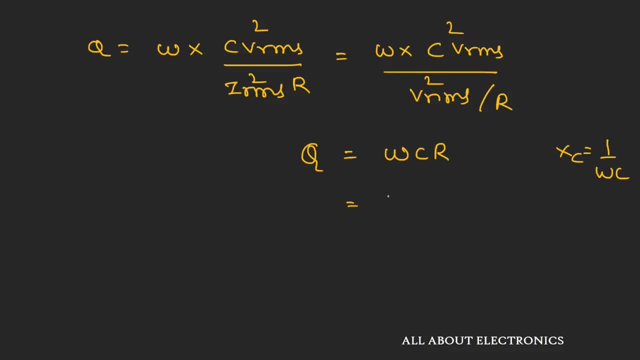 as 1 over Omega C, so we can write this quality factor Q as R over X C, and also, at resonant frequency, the value of X C that is equal to XL. so we can also write it as a R over X L. so this is the equation of a quality factor in terms of. 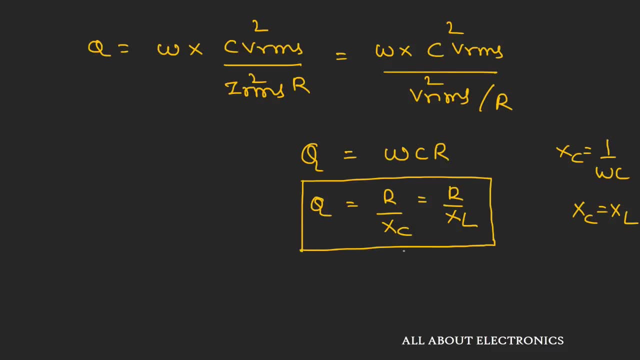 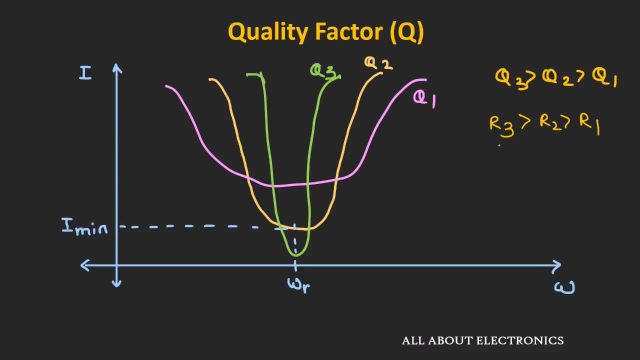 the R over X, L. so this is the equation of a quality factor in terms of the circuit parameters. So now, as you can see here, the quality factor is directly proportional to the value of a resistance. So as the value of a resistance in the circuit increases, 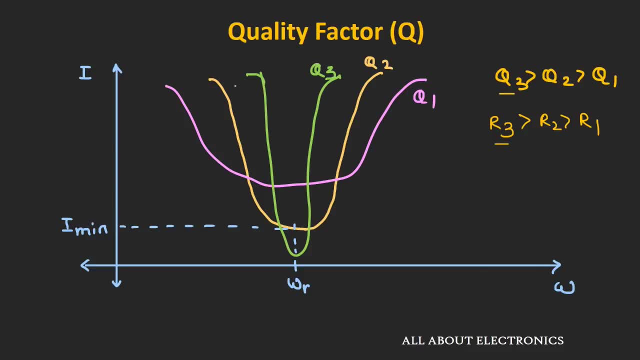 the quality factor will also increase And hence the sharpness of the curve will also increase, And the curve is getting narrower and narrower. And to define how much it is getting narrower we will use the second parameter, that is, bandwidth. So now this bandwidth is defined. 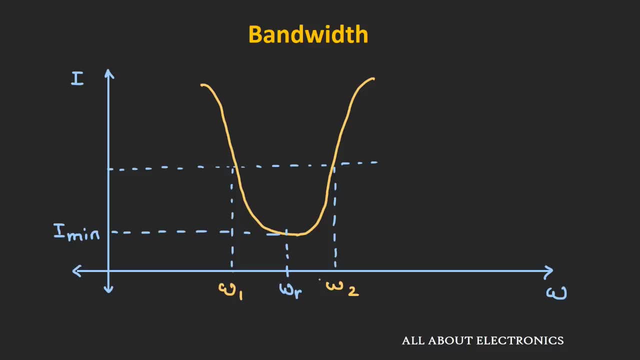 as the difference between the 3 dB frequencies. Now if you see the curve of a parallel RLC circuit at the resonant frequency, the value of the current is minimum. So to get 3 dB point, we will consider the two points where the value of power is doubled. 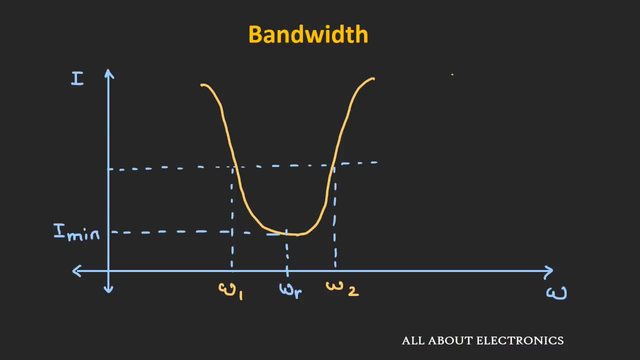 compared to the resonant frequency Or in terms of the current. if we say, the value of current is √2 times the minimum value. So these two points are the points where the power in the circuit is doubled compared to the value of the резonant frequency. 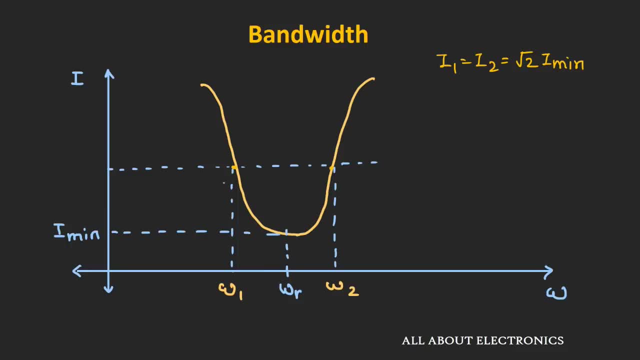 compared to the resonant frequency, Or in terms of the current. the value of current is √2 times the minimum value, And the difference between these two frequencies is known as the bandwidth of this parallel RLC circuit. So now let's derive the expression for this. 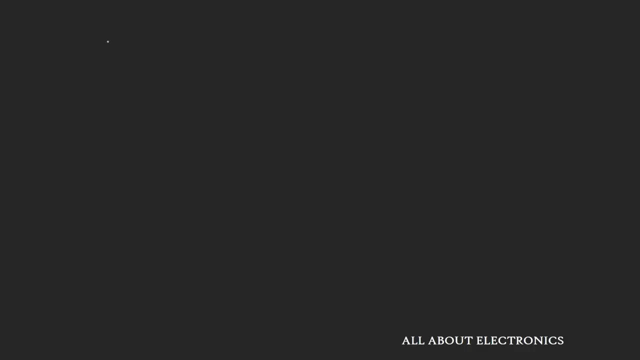 lower as well as the upper cutoff frequencies. So at frequency ω1,, let's say, the current that is flowing through the circuit is I1.. And this I1 can be defined as √2 times the minimum value. Now we can write this current I1 as v into. 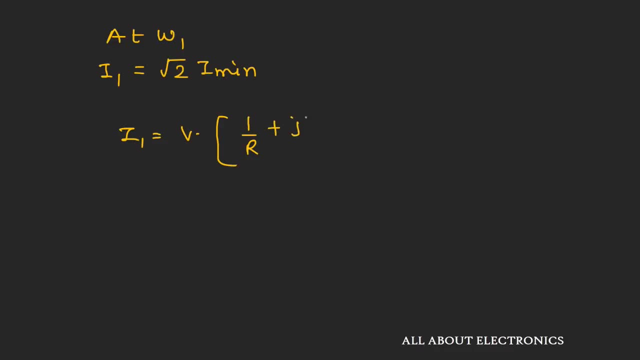 1 over R plus j, into ω1c minus 1 over ω1L. Or we can write it as v into 1 over R, square plus ω1c minus 1 over ω1L, whole square raised to the power of 1 by 2.. 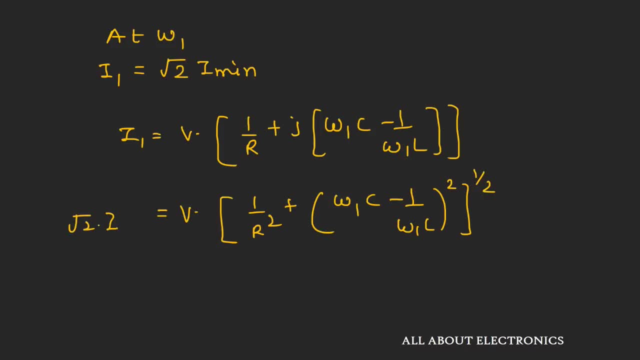 Now this value of I1 is given as √2 times I1.. nothing but root, 2 times i of minimum. And this i minimum is nothing but v over r. So now, squaring up at both the sides, we can get 2 into v square over r, square that. 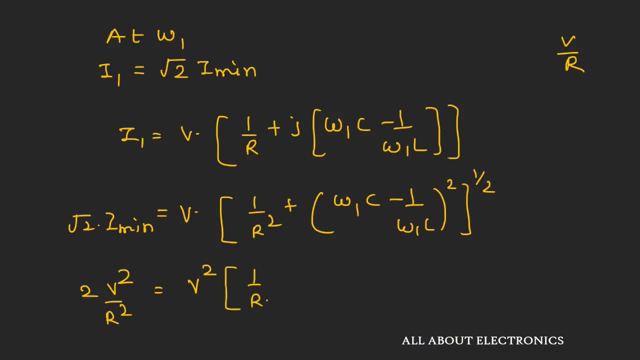 is equal to v square into 1 over r square, plus omega1c minus 1 over omega1l whole square, And if we further simplify it then we will get 1 over r square. that is equal to omega1c minus 1 over omega1l whole square. That means omega1c minus 1 over omega1l. that 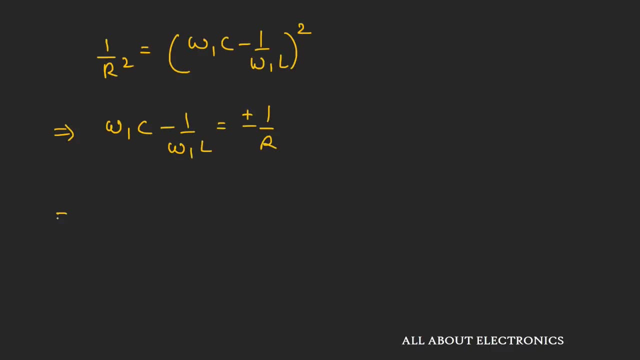 is equal to plus or minus 1 over r. And similarly for the upper cutoff frequency, omega2,. we will get another equation: that is omega2c minus 1 over omega2l. that is equal to plus or minus 1 over r. 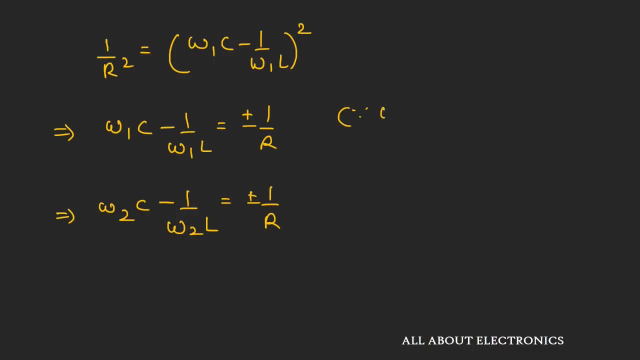 So now we know that this omega1 is less than omegaR and this omega2 is greater than omegaR. Now the frequencies which are lesser than the resonant frequency. if you see, this xc is greater than xl, or we can say that 1 over xc is less than 1 over xl. 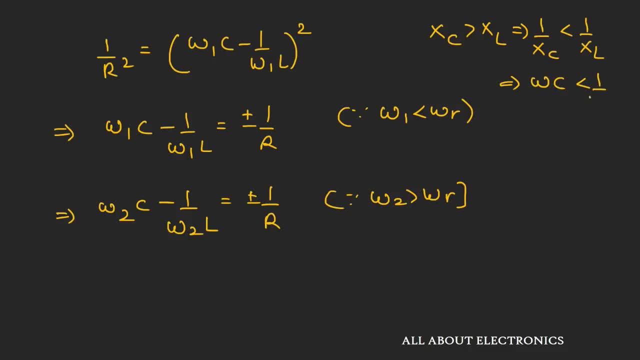 That means omegaC is less than 1 over omegaL. So you see this equation. In this equation the sign of this 1 over r should be negative. That means omega 1c minus 1 over omega 1l. that is equal to minus 1 over r. 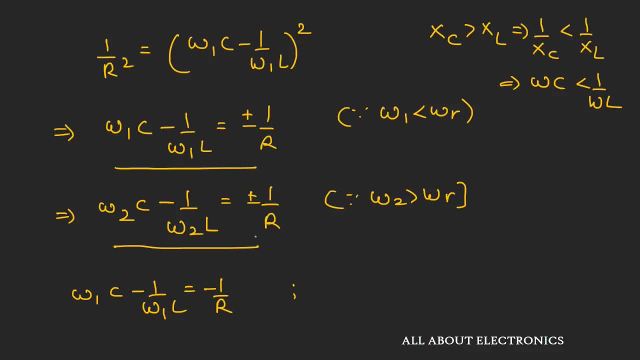 And similarly for this second term. if you see, the omega c will be greater than 1 over omega l, So we will get omega 2c minus 1 over omega 2l. that is equal to 1 over r. 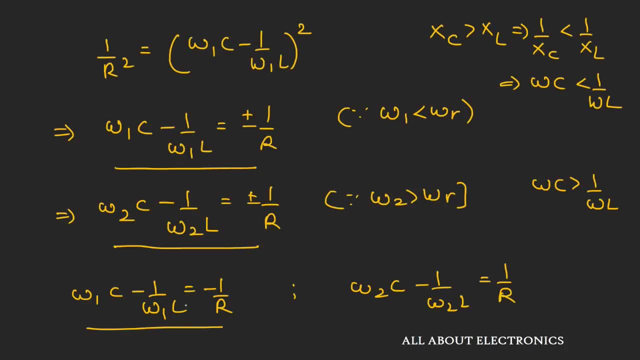 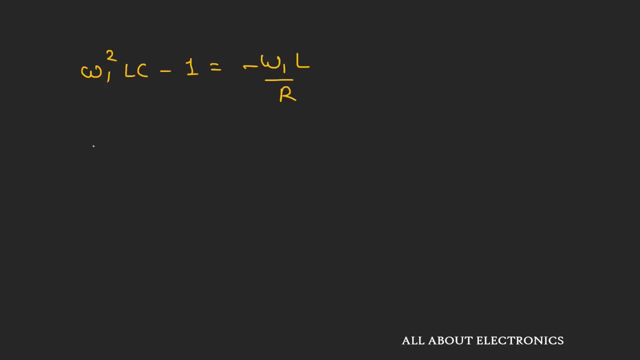 So now let's solve this first equation. So if we simplify this equation, then we will get this equation And further, if we simplify it, then we will get omega 1 square plus 1 over rc into omega 1 minus 1 over lc, that is equal to zero. 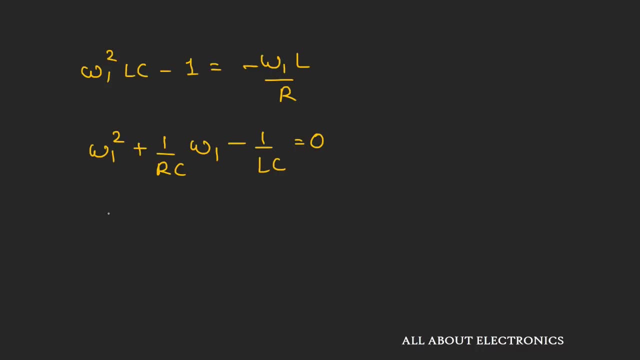 So now this equation will have two roots. So the roots of this equation can be given as minus 1 over 2rc, plus or minus under root, 1 over 2rc, whole square, plus 1 over lc. Now here the frequencies cannot be a negative, so we will only consider the positive term. 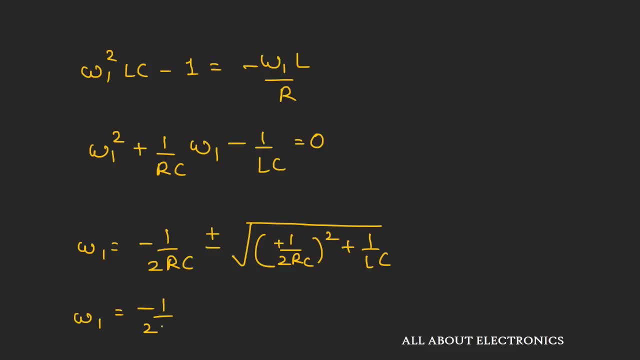 That means omega 1. that is equal to minus 1 over 2rc, plus under root, 1 over 2rc whole square plus 1 over lc, And similarly we can derive the expression for omega 2.. That is 1 over 2rc whole square plus 1 over lc. 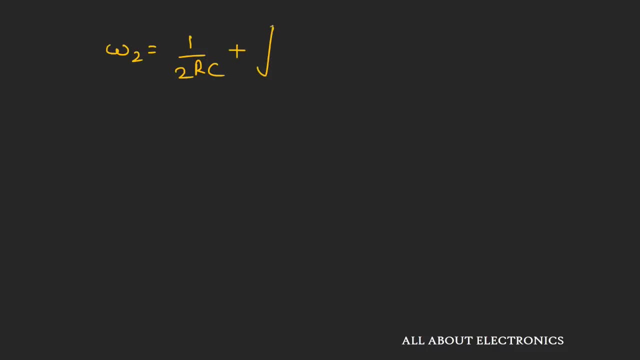 So in this way we have derived the equations for the upper as well as the lower cut-off frequencies. Now, bandwidth can be defined as the difference between this upper and the lower cut-off frequencies. That is nothing but 1 over 2rc, minus, minus of 1 over 2rc. 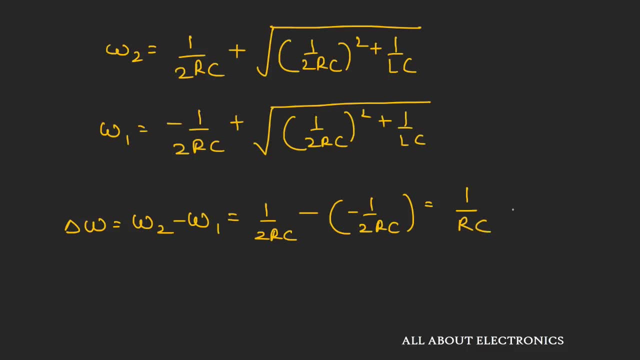 That is nothing but 1 over 2rc. Ok, So in this way the bandwidth can be defined as 1 over rc. Now, if we multiply these two equations, then we will get omega 1 into omega 2. that is equal. 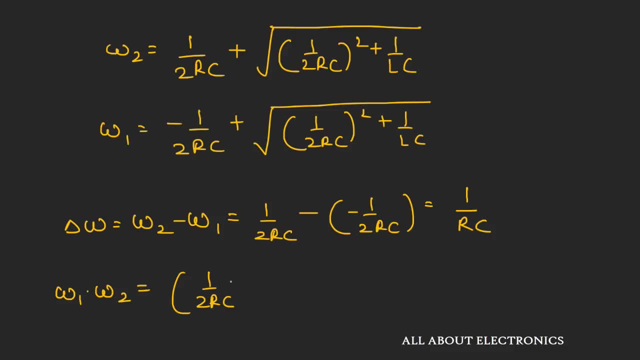 to 1 over 2rc whole square, plus 1 over lc, minus 1 over 2rc whole square, That is equal to nothing but 1 over lc. So in this way we will get omega 1 into omega 2.. 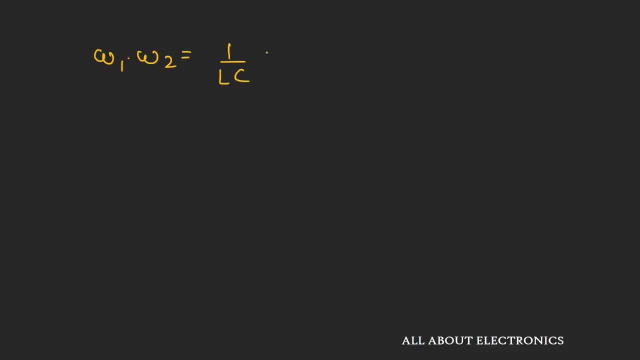 So in this way we will get omega 1 into omega 2 as nothing but 1 over lc, And this 1 over lc is nothing but omega r square, That is the square of the resonant frequency. So in this way omega r can be written as under root: omega 1 into omega 2.. 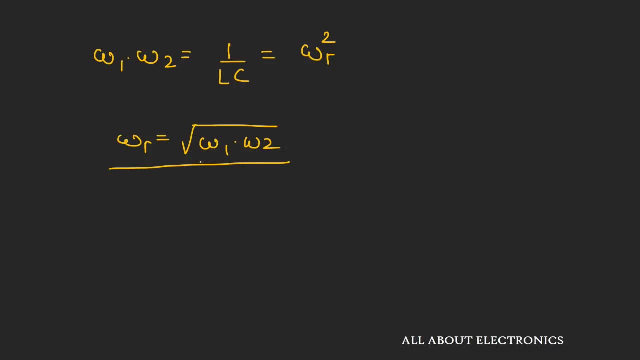 So this is nothing but a relationship between the upper and lower cut-off frequencies with a resonant frequency. So earlier we had found out the equation for the quality factor Q as nothing but r over lc, That is, r into omega c. Now here, according to the equation of bandwidth, delta omega is nothing but 1 over rc. 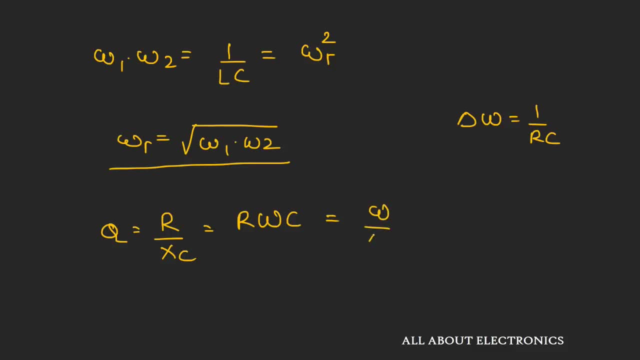 So we can write this equation as omega over delta omega, which defines the equation between the quality factor and the bandwidth. That means Q is nothing but omega over delta omega. Also, if you see this, Q is nothing but omega into Cr, where omega is nothing but a resonant. 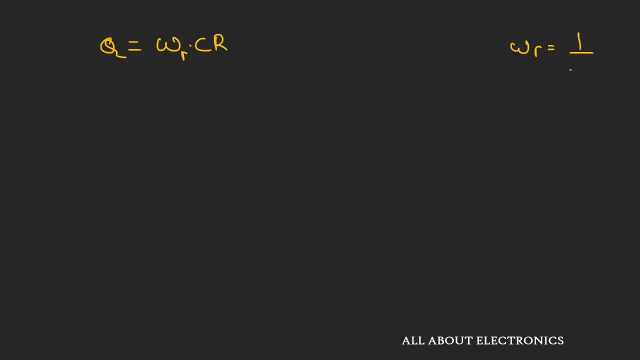 frequency quarter, and gt is only left as mass per sagt, And we know that omega r is nothing but 1 over under root lc, So we can also write this quality factor Q as under root c over lc into r. So this is how this quality factor can be defined in terms of the circuit parameters. 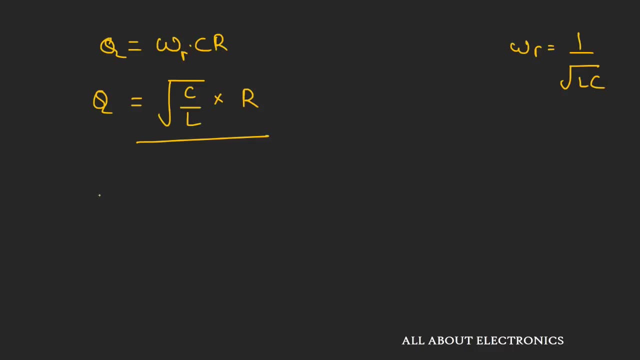 So now at resonant frequency, if you see the inductor current, Il can be defined as v over xl. So now at resonant frequency, the voltage v can be written as il into cuánta 1rc divided by xl. 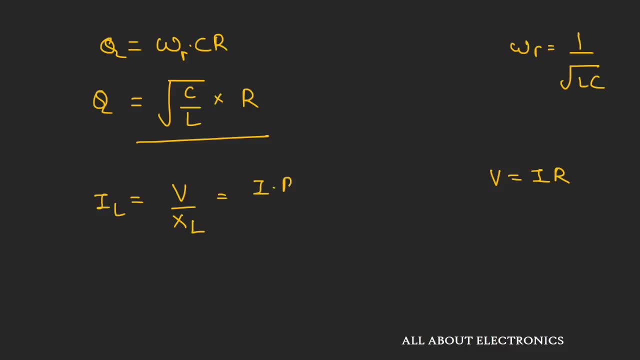 into R, That is, I into R divided by xL. And if you see this term, this term is nothing but a Q, So we can write this inductor current I as nothing but a Q into I. Similarly, if you see, 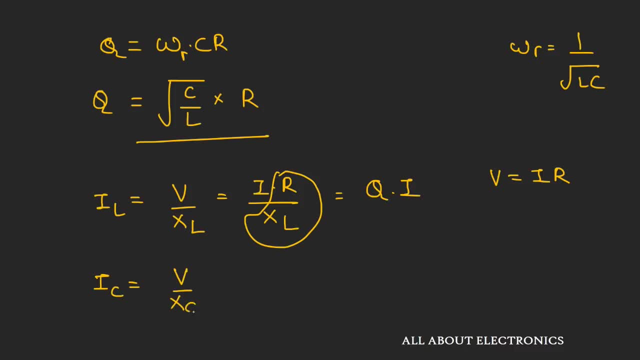 the capacitor current, which can be written as V over xC And we can write it as I into R over xC. Again, this term is nothing but a Q into I. So in this way, if you see, at resonant frequency,